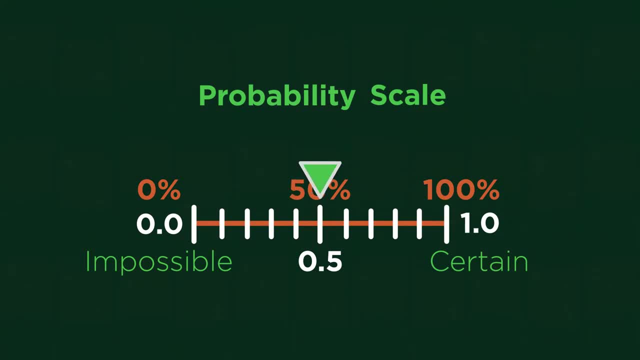 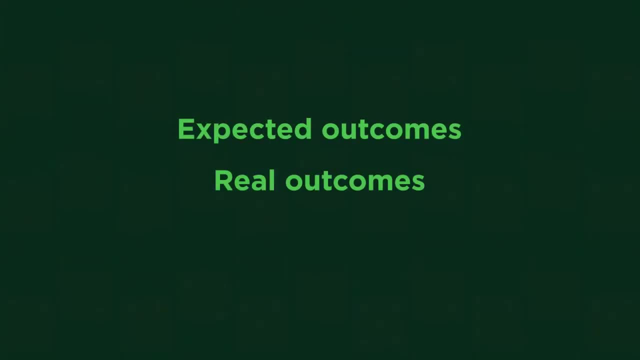 anywhere on the scale, with a 50% chance in the middle. Another use of probability is to distinguish between expected outcomes and real outcomes. For example, tossing a coin, You expect that there is an even chance of getting heads or tails. The probability of getting heads in this case would be the ratio between the 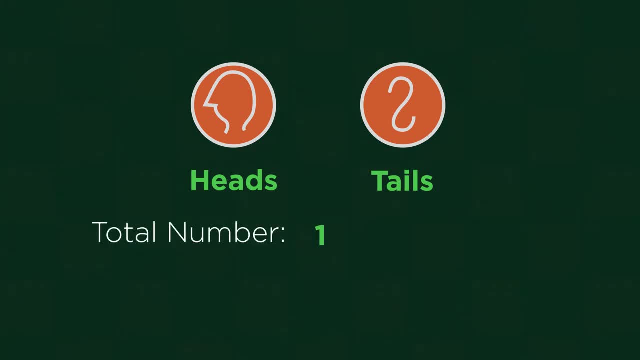 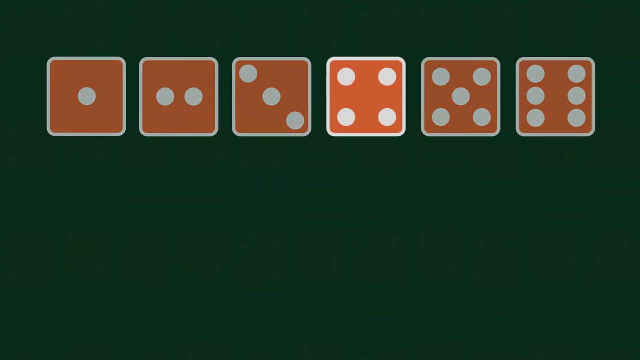 number of times- that is one- you can get heads and the total number of outcomes, that is two. That means that the probability of getting heads when tossing a coin is one over two. If you roll a dice, there are six possible outcomes and the chance of getting heads. 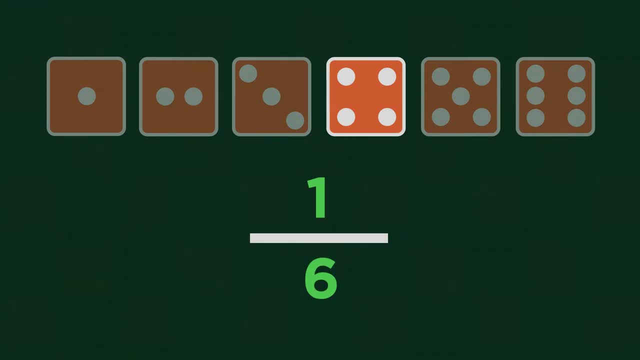 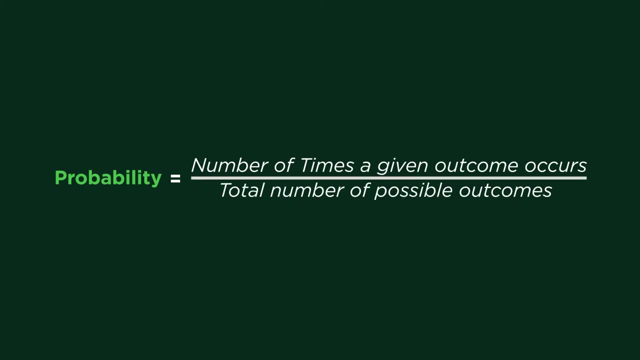 is one out of six. Remember this formula to help you do the calculations: Probability equals the number of times a given outcome occurs over the total number of possible outcomes. Sometimes it will occur that it is difficult to find the probability of an event happening. 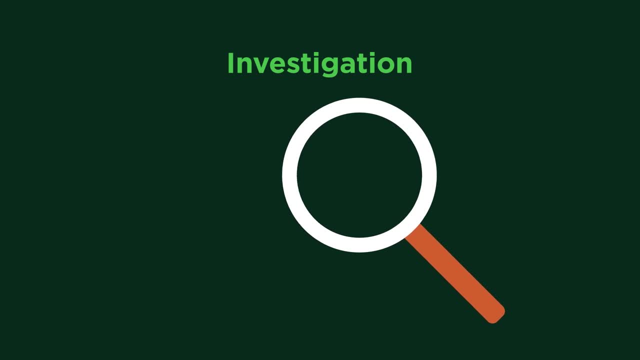 You can then do an investigation to calculate probability. When investigating, you compare the real outcome of a given event with the total number of possible outcomes. This can be done by calculating the relative frequency of a given outcome. The relative frequency of an outcome is the ratio between the number of outcomes obtained. 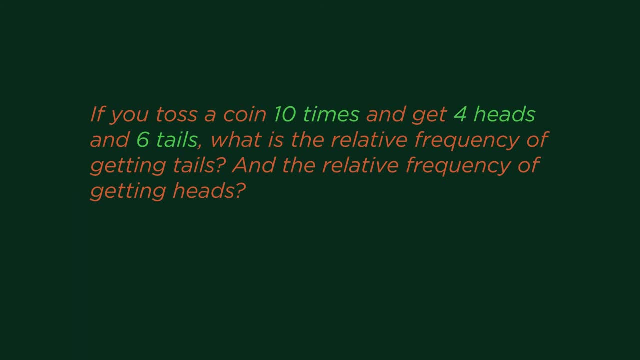 and the total number of possible outcomes. Try this: If you toss a coin ten times and get four heads and six tails, what is the relative frequency of getting tails and the relative frequency of getting heads? Pause the video while you work it out. 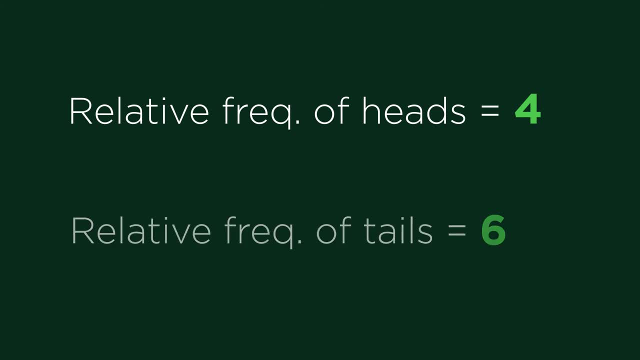 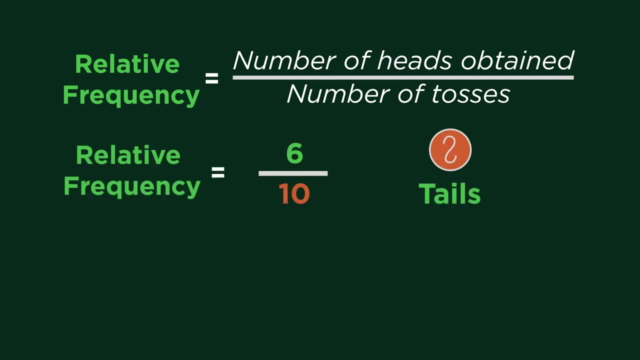 Well, the frequency of heads is four and the frequency of tails is six. so we use the following method to help you calculate: Relative frequency equals the number of heads obtained over the number of tosses. That means the relative frequency of getting tails is six. 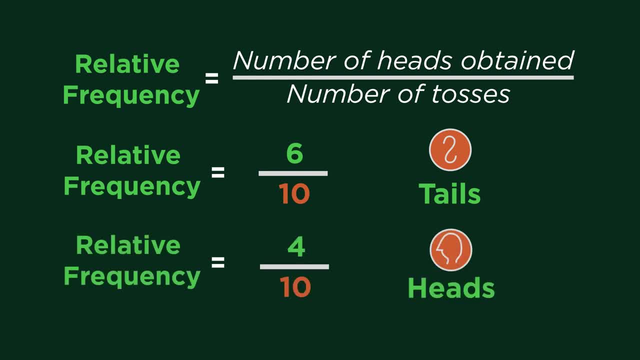 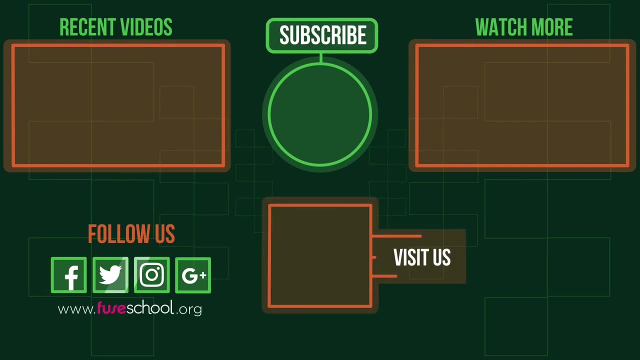 out of ten and the relative frequency of getting heads is four out of ten. Now you know three ways of how probability experiments can be done. If you liked the video, give it a thumbs up and don't forget to subscribe. Comment below if you have any questions. Why not check out our Fuse School app as well? Until next time.